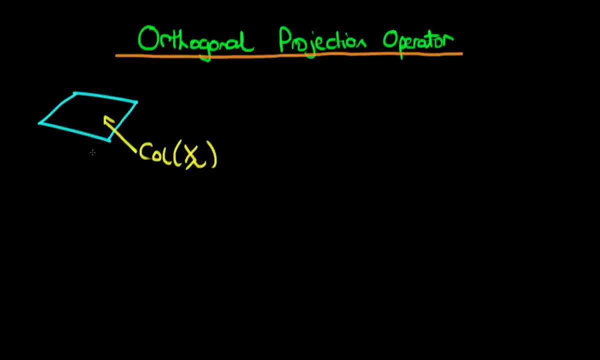 x and that defines a particular plane in some sort of higher dimensional space. And the idea is that we're trying to get as close to y, which lies off of that column space in terms of a particular, by choosing a vector which lies within that column space, which we're calling mu hat. 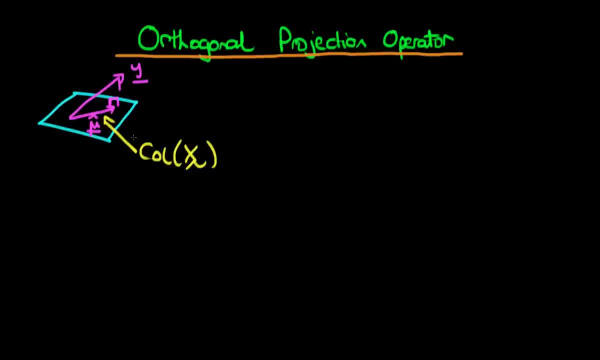 And I've sort of mentioned in passing that mu hat really represents the orthogonal projection of y onto the column space of x. So in this video we're actually going to define what actually do we mean by the orthogonal projection operator and how do we actually go from y to mu hat. 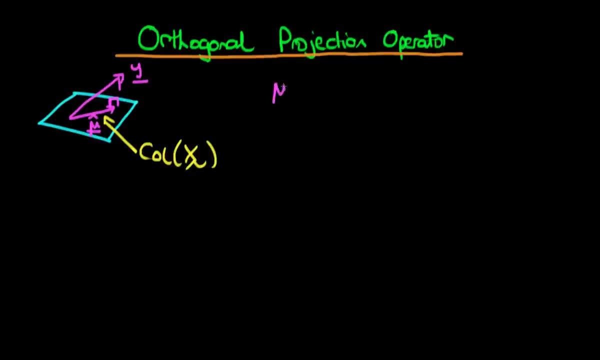 Well, we can actually already answer this. We know that mu hat is just given by x times beta hat. And since we know that beta hat is x primed x, all to the power minus one times x primed y, then we have an expression for mu hat in terms of y. 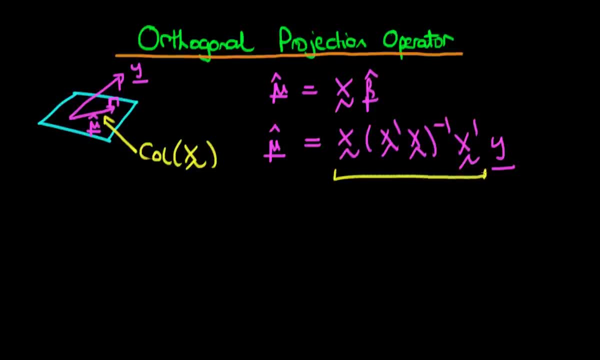 So sense would seem to suggest that this sort of term, which I'm underlining here, really is the orthogonal projection operator Which transforms y or projects y onto the column space of x. So we call that orthogonal projection operator px and we just let it operate on y. 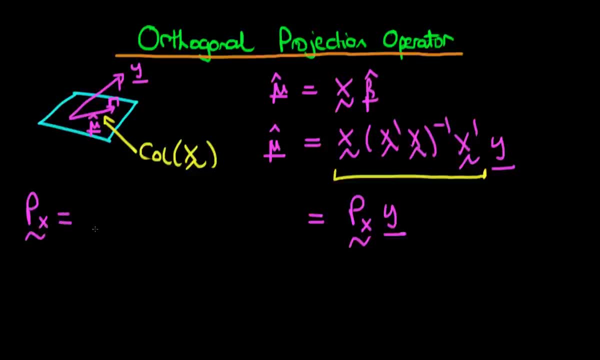 So, from the logic which we've used thus far, we can identify that px is actually equal to x times x primed, x to the power minus one times x primed. Okay, and we can ask what sort of properties this projection operator should have. Well, if we were to choose any vector which lies within the column space, 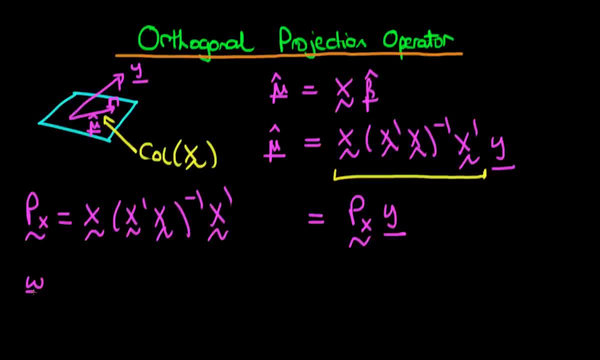 So let's assume we picked a vector- let's call it w- which lies within the column space of x. Then if we apply the projection operator to that vector w, then we should just get that original vector w out in the first place, because the projection of a vector which already lies 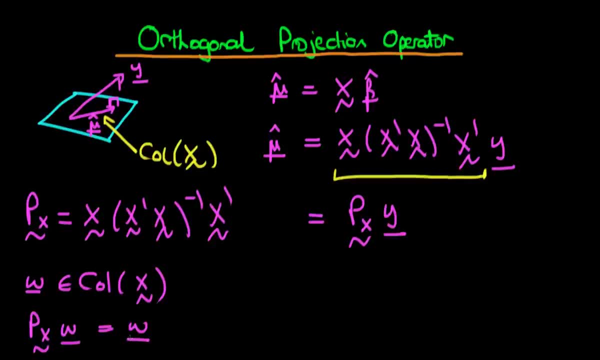 onto the columns in the column space is just going to be itself. You can't get any better projection than that. Similarly, if we have a vector w which is at right angles with the column space of x, Then we should expect that p of x times w should be equal to zero, because there is no way for us. 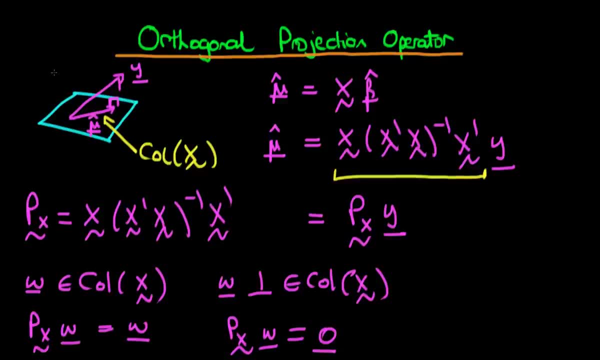 to project down that particular vector. You imagine a vector w which looks something like this. Then there's not actually going to be any projection of w onto the column space of x. Okay, so let's try it out a bit. then We know that the vector mu hat lies in the column space of x. 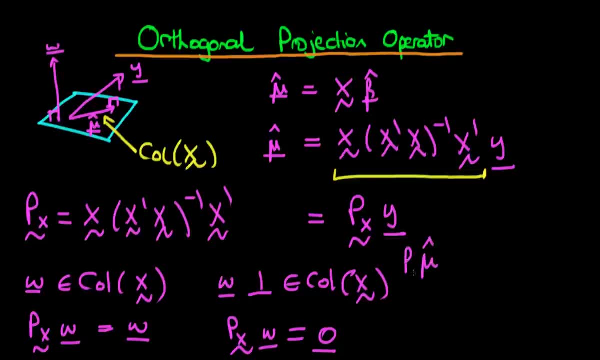 Hence we expect that mu hat. if I use the projection operator on mu hat, then I should just get mu hat out in the first place. Actually, I'm running out of space a little bit here, so I think I'm actually going to continue this on in the next video and we're going to show that the projection operator 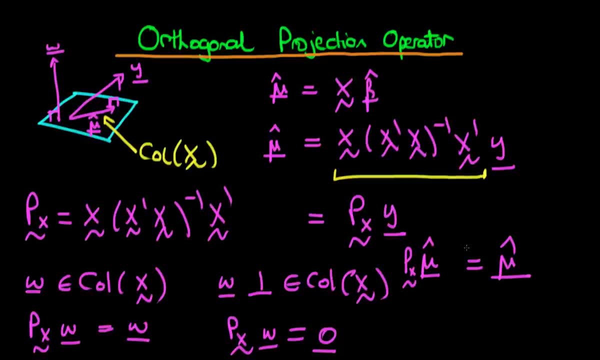 actually has the or the orthogonal projection operator actually has the properties which we expected to have? 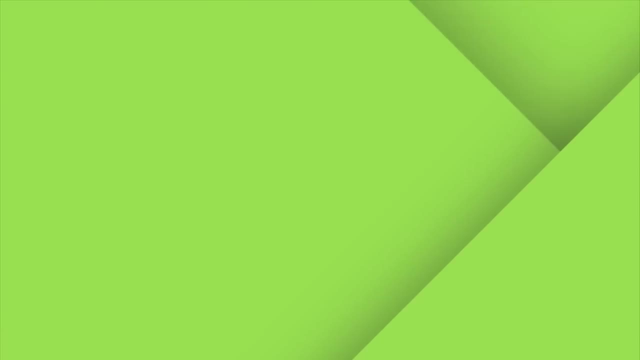 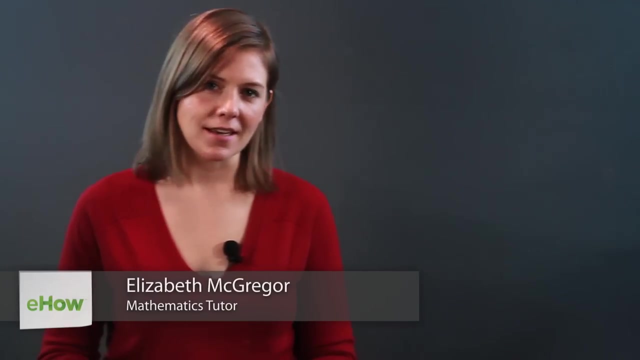 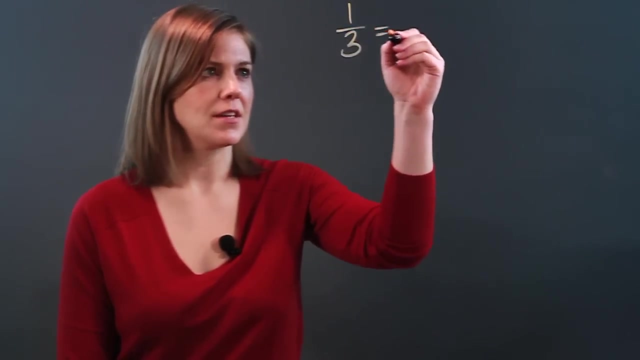 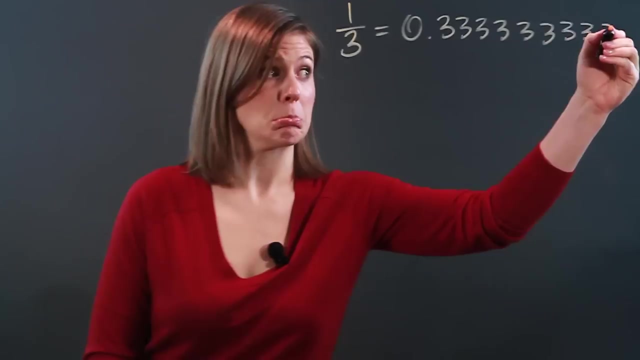 Hi, I'm Beth. I'm a math teacher and I'm going to talk to you about the difference between a repeating decimal number and a terminating decimal number. It's pretty clear once you see it. One third is a fraction that, when written in decimal form, is 0.3333333 repeating. 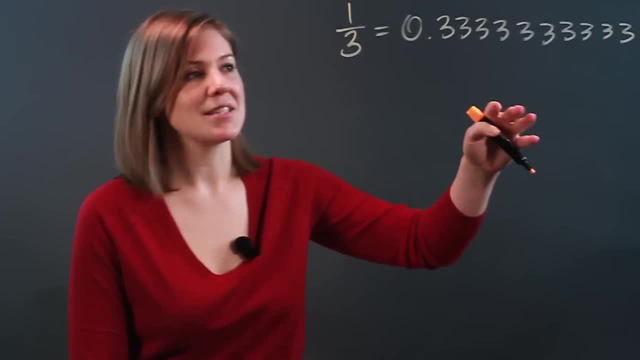 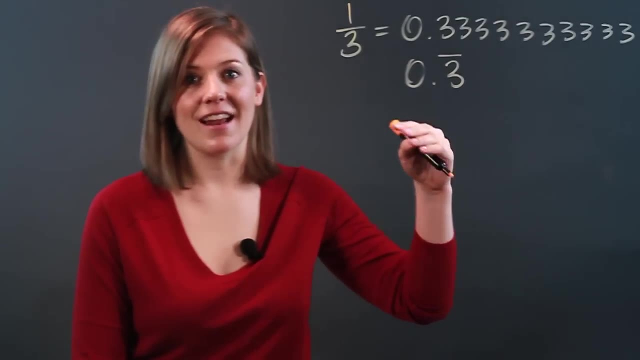 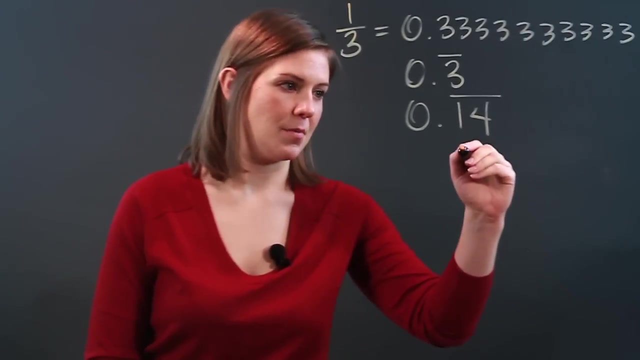 straight off the board to infinity. Any sort of repeating decimal will have a period. Here the period is just 3, because the 3 is what repeats. You might see in other numbers that it might be .14 and the 14 continues to repeat, which would be equivalent to 141414.. So those 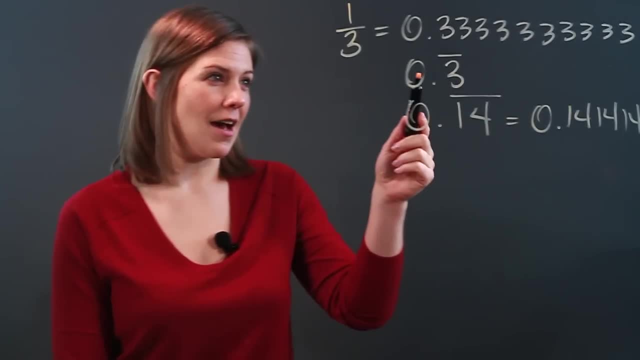 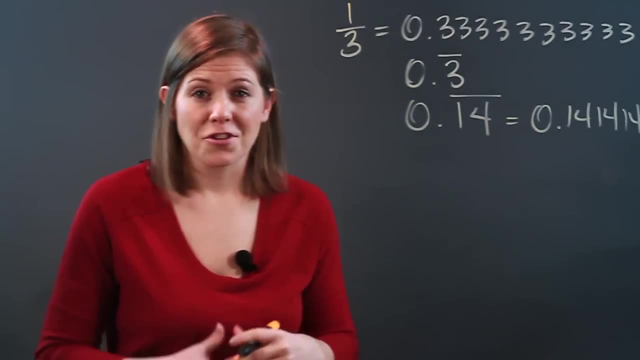 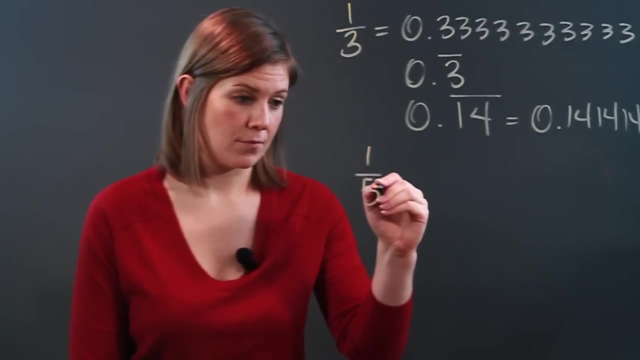 are both repeating decimal numbers. You might say that like 0.3 recurring or 0.3 repeating. Now, in terms of a terminating decimal number, terminate means end, So it's a decimal that has a clear end. A great example: one half. Oh, I wrote one fifth, I was getting ahead. 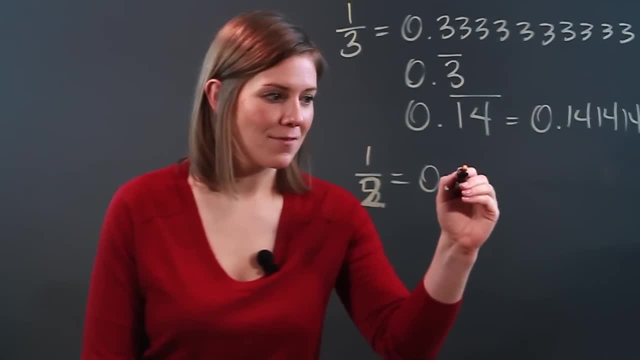 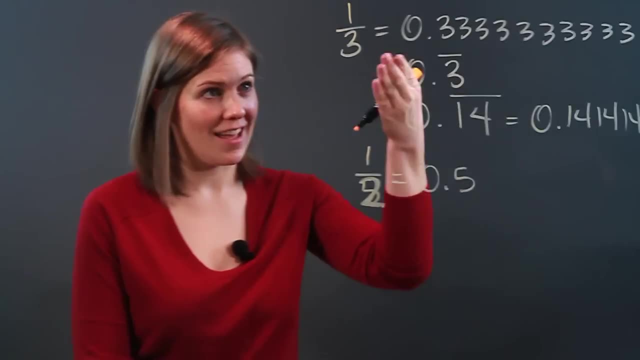 of myself. One half equals .5.. It terminates The end. That's it. That's all you get, And that's a good example of a terminating decimal. One third is a good example of a repeating decimal number, both of which are rational numbers. 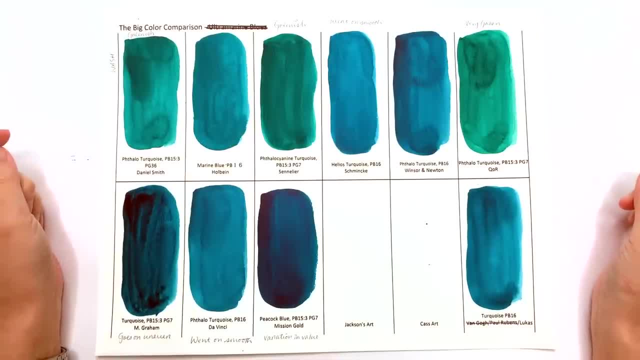 Welcome to episode 2 of the Colossal Color Comparison series. In this episode, we're going to be taking a close look at phthalo turquoise. The last episode ended up being 30 minutes long and I totally realized that that's way too long.